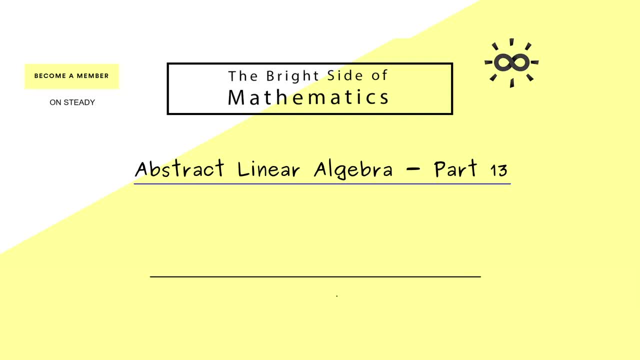 to explain why orthogonality is so important for us, Just imagine a straight line and a vector x which is not parallel to this line. Moreover, if you imagine that the sun shines from top to bottom, then this arrow would make a shadow here on this line. And indeed, if the sun shines from the top, 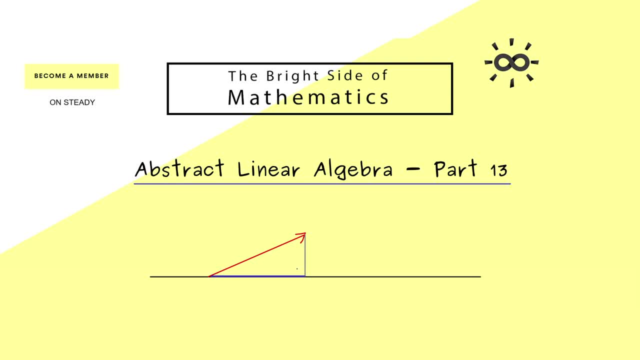 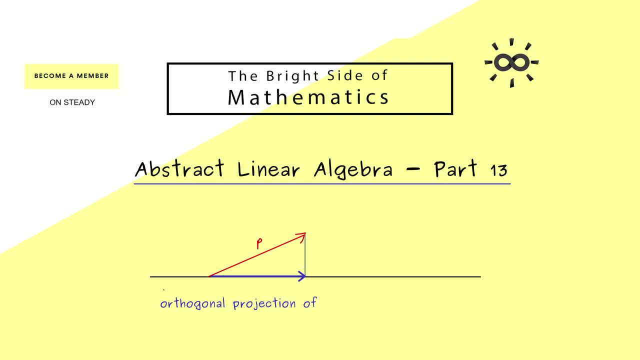 The orthogonal projection of P. More precisely, it's the orthogonal projection of the vector onto the subspace given by this line. And you see in the picture that this orthogonal projection is also a vector. But this is not all, because we also find a third vector here. 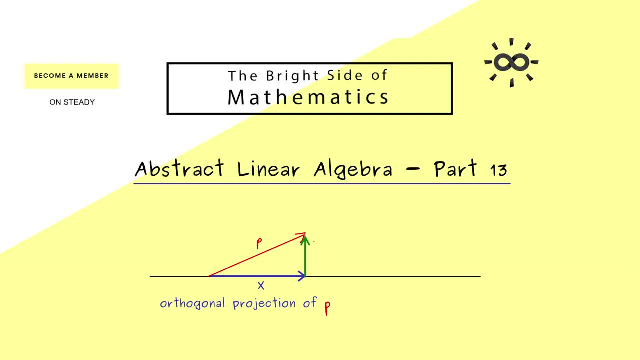 which we could call the normal component of P. And again, this is with respect to the given fixed subspace. here And again, this is with respect to the given fixed subspace. here And again, this is with respect to the given fixed subspace here. 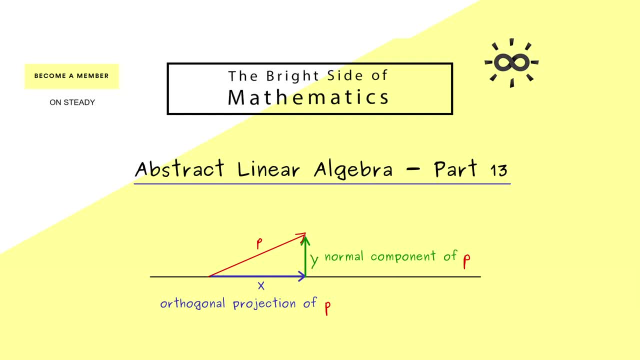 And now, if we call this vector y, we have a linear combination for P, Namely: P is given as x plus y. Now, of course, this is not a surprise, because you can always decompose a vector into a linear combination. 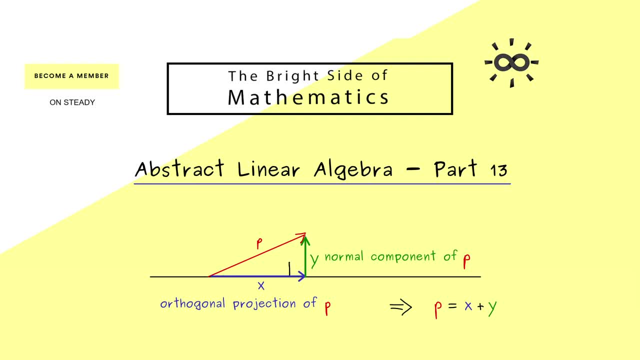 However, here we want more, because we want to have a right angle between x and y. Of course, this is exactly what orthogonal means here. However, this right angle here should be seen in a general context. It's a general right angle, which means: 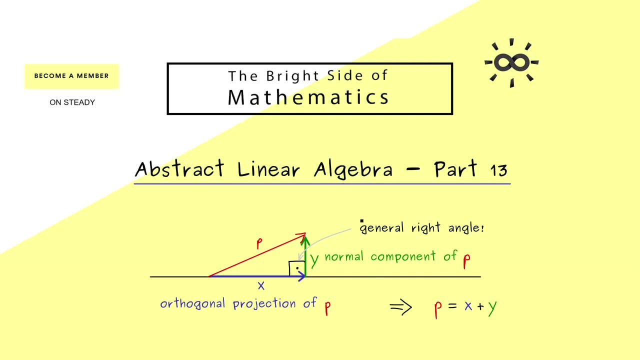 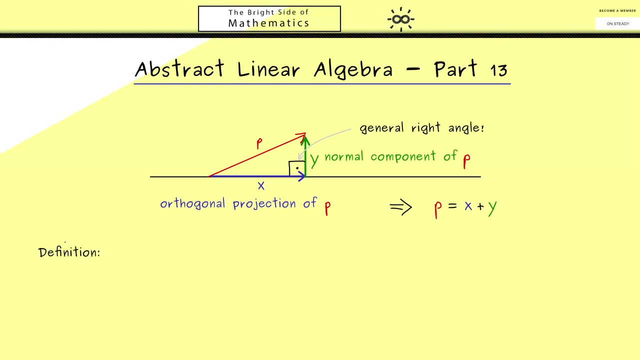 it's only given by our inner product. So you immediately see this is a general and important concept we should put into a formal definition. In other words, it's not a problem at all to generalize our picture here. However, the general definition of an orthogonal projection, we will do. 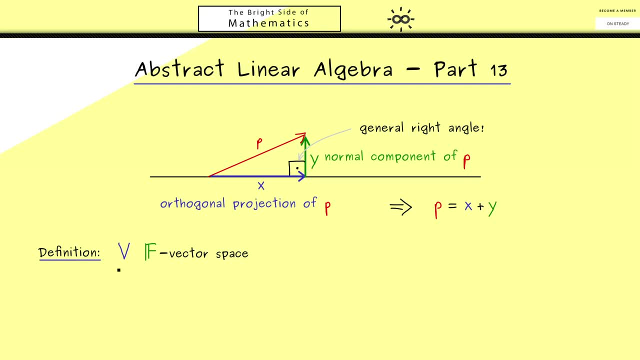 in the next video. Here we first define the basics, and for that, as always, we need an f vector, space v and an inner product. An inner product is always denoted with the pointed brackets here, and you know, we have three properties. And now we say that two vectors, x and y, are orthogonal. 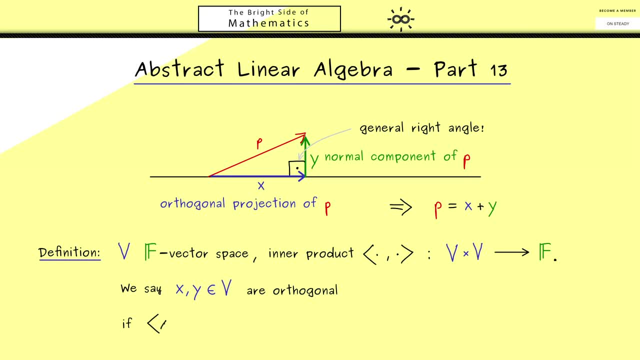 if the inner product of x and y vanishes. This should not be a surprise for you, because this is exactly what we want to do in the next video: What we have for the standard inner product in Rn, And now we just generalize that for any inner 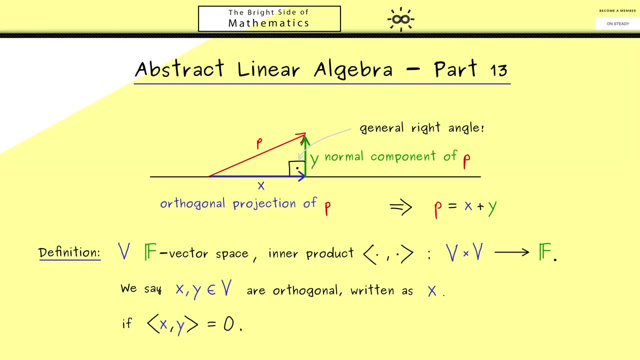 product we can have. Moreover, we also use a common symbol here to denote that two vectors are orthogonal. So please remember: the symbol here simply means that x and y in the given inner product give us zero. So you see, this is not complicated at all. and in the picture above 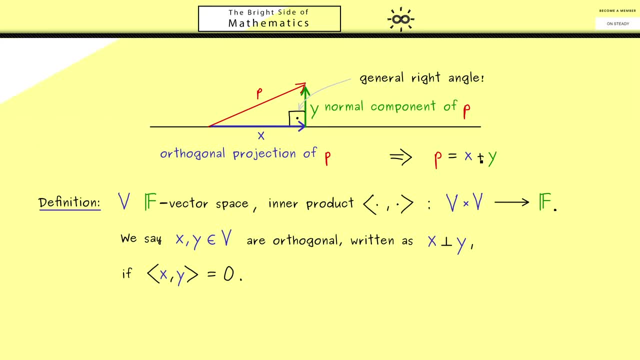 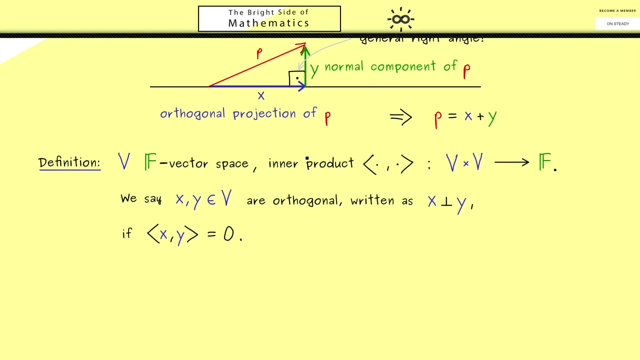 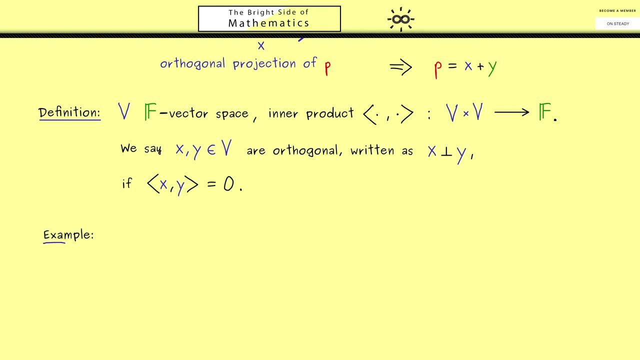 you see, we want that x and y in the inner product give us zero. So we could say the picture looks always the same but the interpretation, the meaning is different depending which inner product space we have. So for example, we could look at a polynomial space. again, Let's take the polynomials that are defined on the 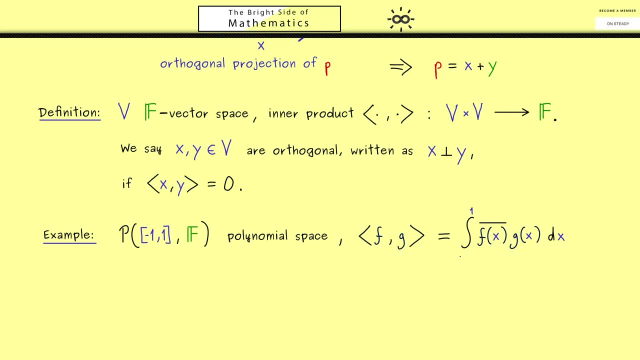 interval minus one to one And then, as we have discussed in part 10, a possible choice for an inner product. is this integral? here And now, we can just take some simple polynomials and maybe let's call them p1 and p2. And an easy choice would be monomials. 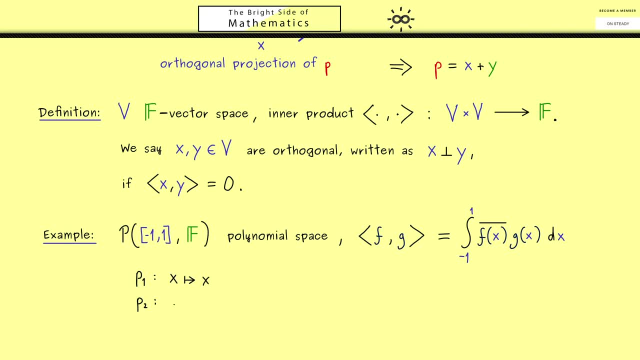 So let's say p1 sends x to x and p2 should send x to x squared. Then we can just calculate the integral here. This is not complicated at all, because we just have to integrate x cubed, which gives us by a symmetry argument immediately zero. 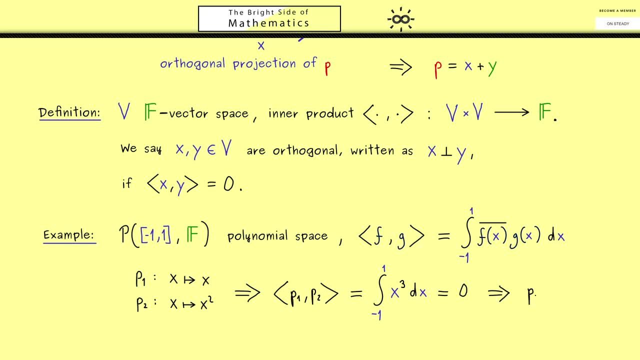 Hence p1 and p2 are orthogonal. This means, if we see the polynomial space here with the geometry given by the inner product, then p1 and p2 have a right angle in between. So what we take from that is that the term orthogonal now also makes sense for polynomials. Indeed, 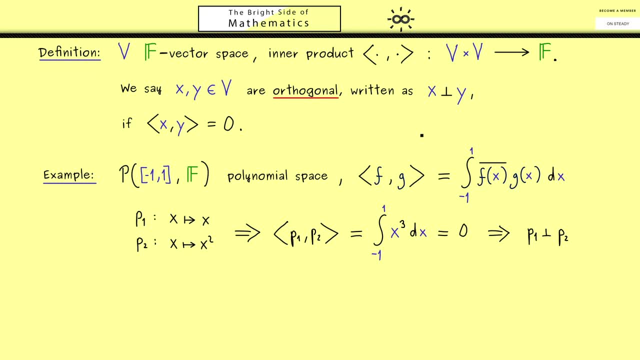 the only thing we need for this term is an inner product space, which is simply any F vector space with an inner product. okay, then let's talk about another important definition here, which is about the orthogonal complement. the assumptions we need here are the same as before, so vector space together with an inner product. and now 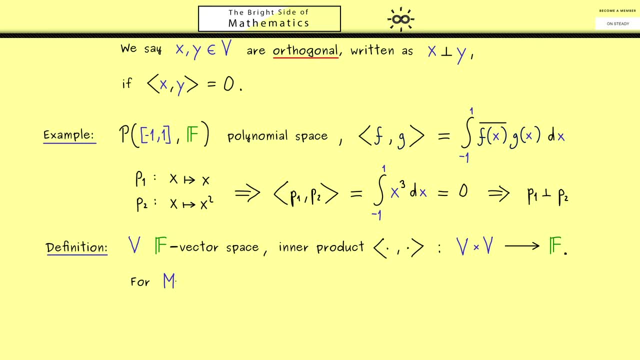 for any subset M in V, we can define the orthogonal complement of M. however, usually we exclude the empty subset from this definition. so you see, M does not have to be a subspace at all. it's enough that we have a subset of the vector space. however, I can already tell you that the resulting orthogonal complement 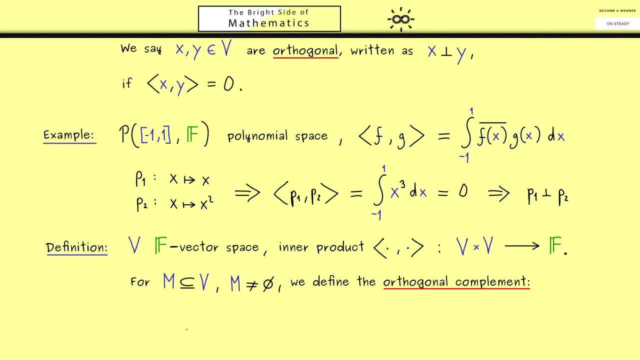 is a subspace and the common notation one chooses is M, together with this perpendicular symbol. so the same as before, but now as a superscript. so you might already guess that the definition is not so complicated, because we just take the set of all vectors- and maybe let's call them X here- that are perpendicular to all vectors from M. 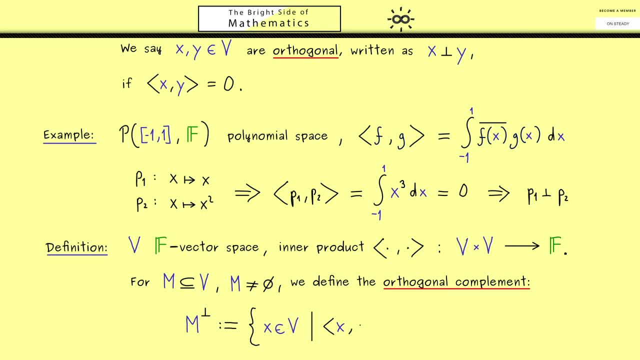 hence we can write X in the inner product with a vector. M is equal to 0 for all M in M, and this is already the whole definition here. so you see, we just take all the vectors X in V that go into the orthogonal direction of M. so for 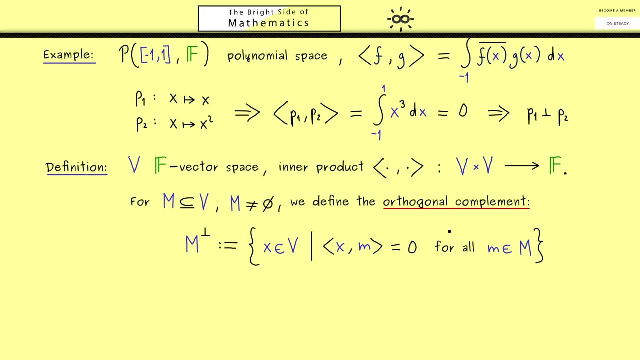 example, you can visualize the set of all vectors, X in V, that go into the orthogonal direction of M. so for example, you can visualize that in R3 by taking M as a line, and if that's a line through the origin, then M has only one essential direction and then the orthogonal complement of M is a. 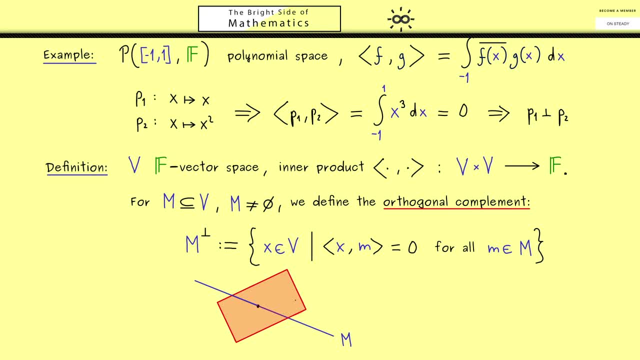 whole plane in R3. this means any vector from this plane is orthogonal to all the vectors in M. and of course it's even easier to visualize if you don't take the whole space R3 but just the plane R2. then if you have a line through the origin, again the orthogonal complement. 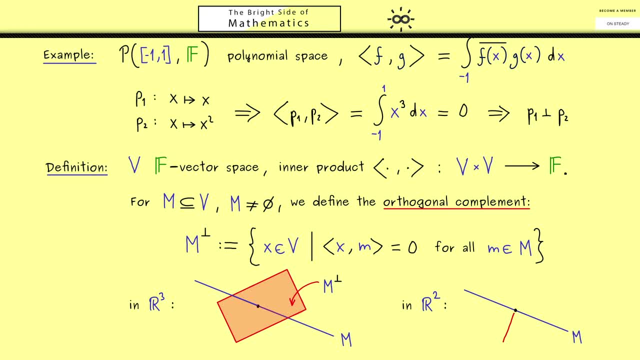 will be a line as well, and obviously it has to be the orthogonal direction here. moreover, something you might immediately notice here is that in the case that M is a subspace, we have that the dimension of M plus dimension of M orthogonal is equal to the dimension of the whole space. so you see, in this sense, the